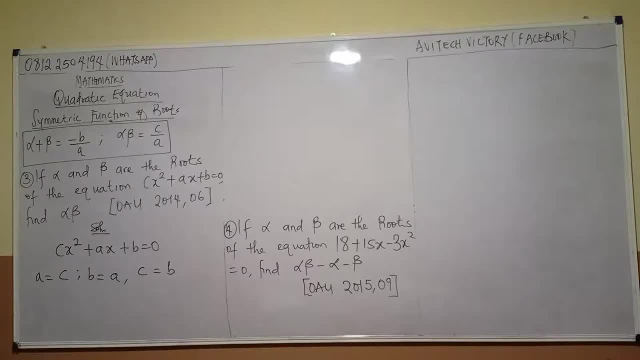 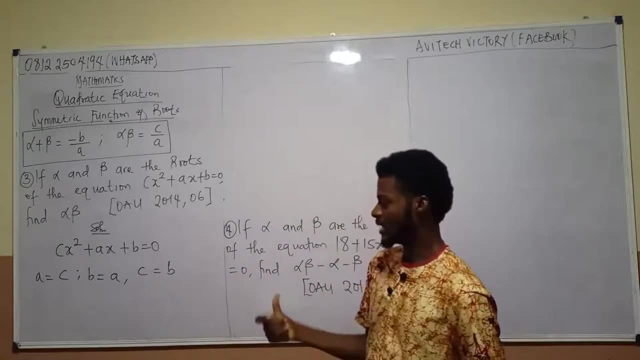 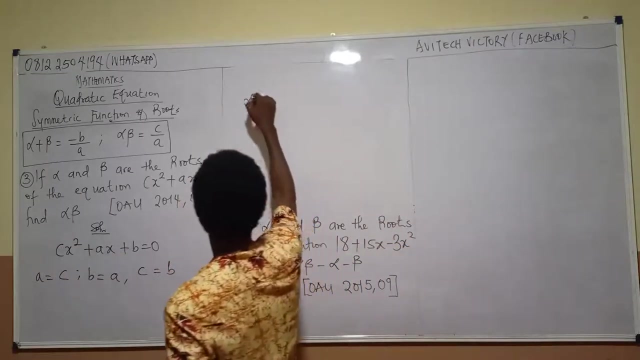 B is the number with X, YC is the number with what, Without anything. Now look at this: If A is C, B is A, C is B. The question says: find what Alpha beta. So what did I say? is alpha beta? 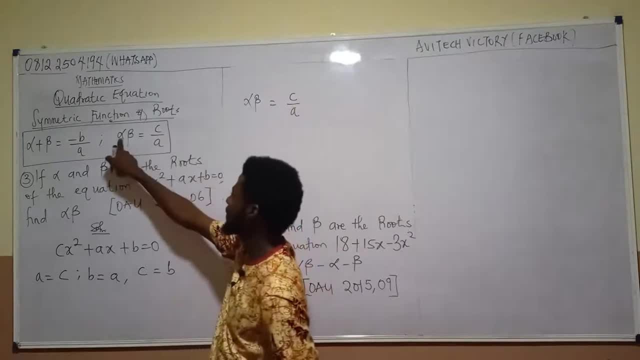 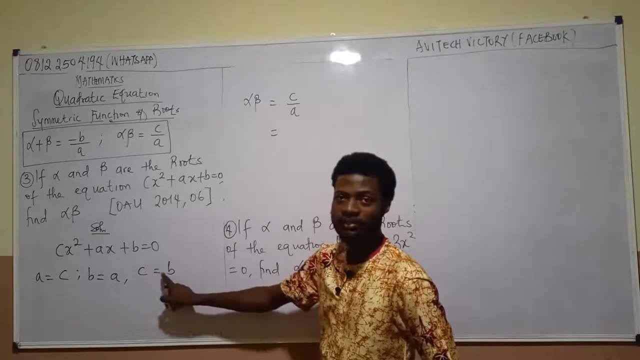 Alpha beta is C over A. Look at it here: Alpha beta is what C over A. So right now, what is C in the question? C is equal to what B, C is equal to B. So this is B over what is A. 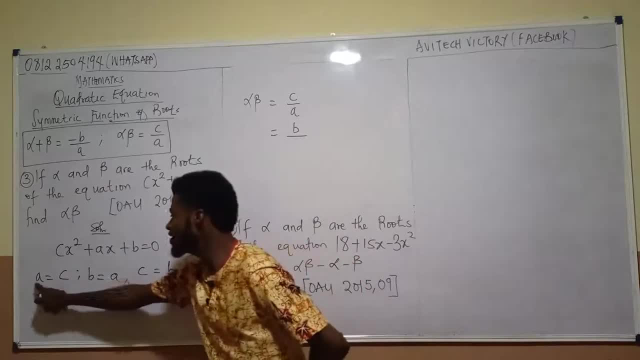 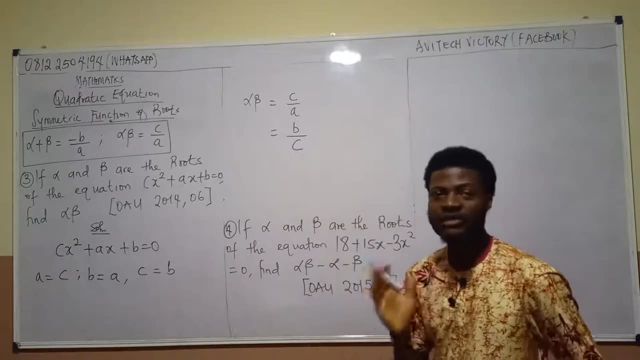 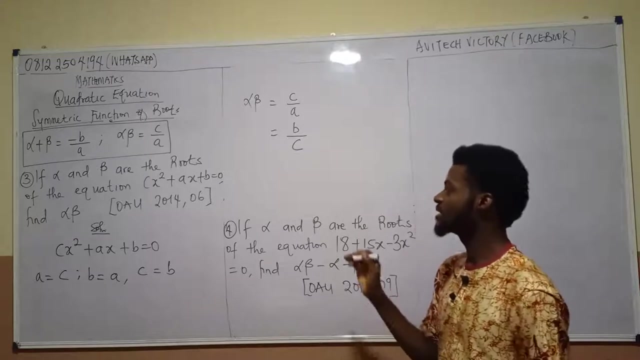 in the question. A is what C. A is equal to C, So the answer for this question is B over C. It's quite simple, but a person might make some silly mistakes. But the answer is: what B over what C? That's the answer. 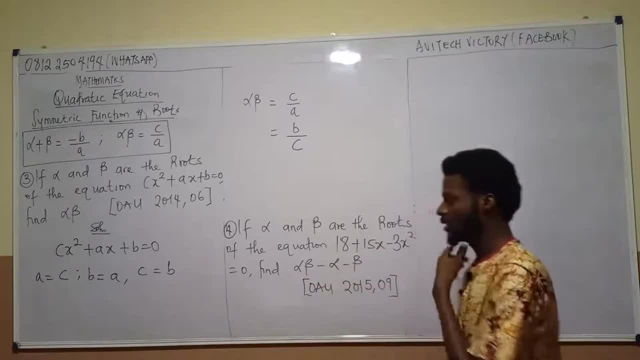 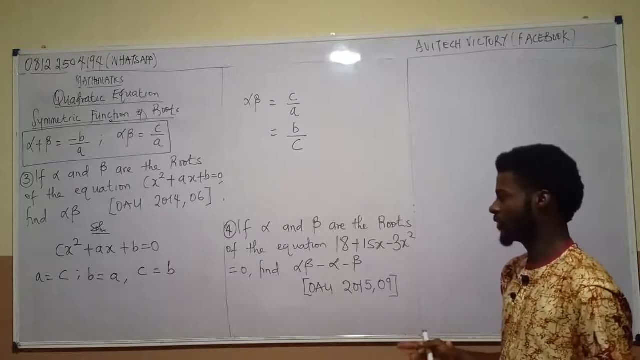 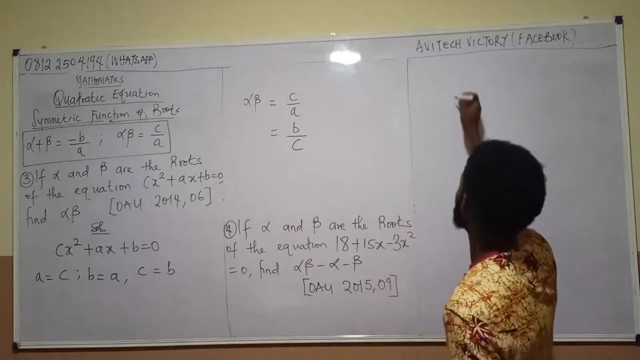 So if this is the answer to the question, let us proceed to the next one. Let us proceed to the next one. The next one says: if alpha and beta are the roots of the equation, 18 plus 15X, take away 3S squared equal to zero. The first thing you do is to write that out: 18 plus 15X. 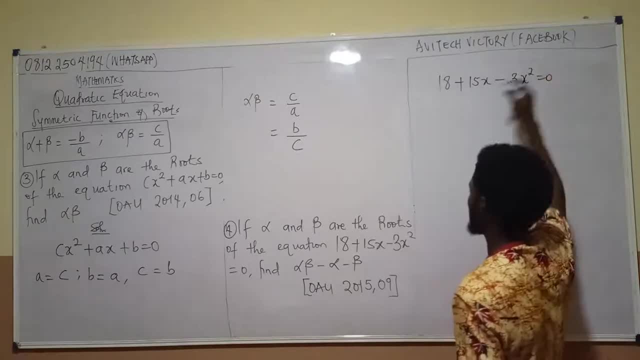 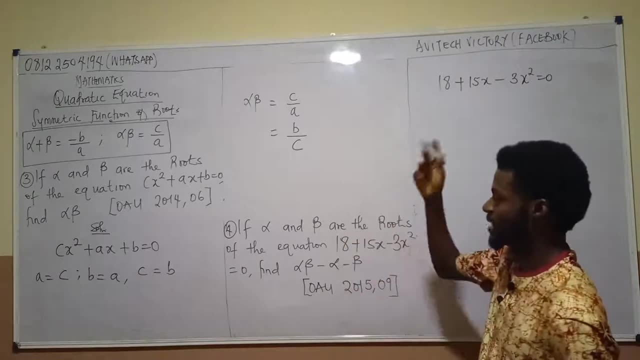 take away 3S squared equal to zero. That's the first thing you do, But the next thing is this: The next thing you do is this: Bring out A, B and C, So A will be equal to something. Now remember. 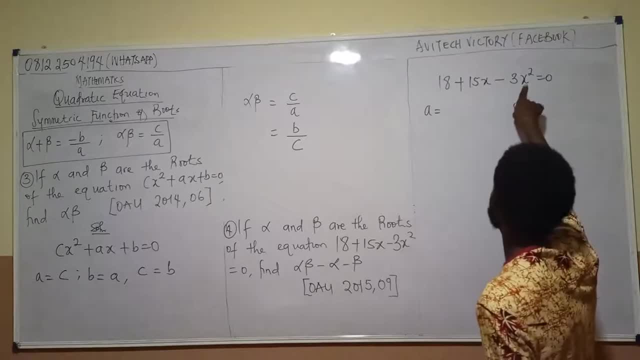 A is the number which was S squared. So what is this S? What's the number which is minus 3? Minus 3.. So this is minus 3.. The word is B. B is the number with X, So that's 15.. The word is C. C is the constant without an. 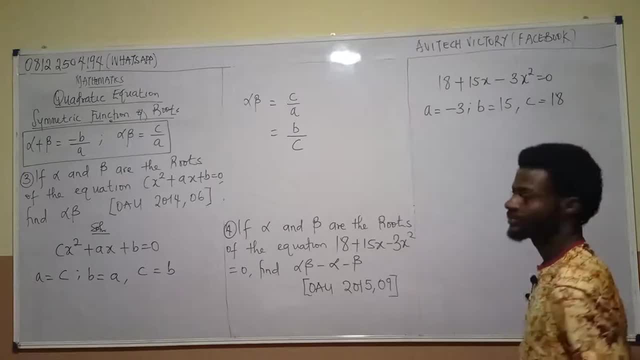 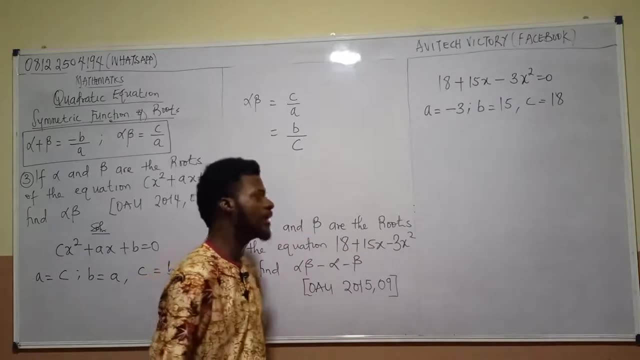 alphabet. So that's what, 18.. Now, if A is minus 3, B is 15,, C is 18.. The next thing is: what would then become alpha plus beta and alpha beta? You don't just start solving this right away. So if 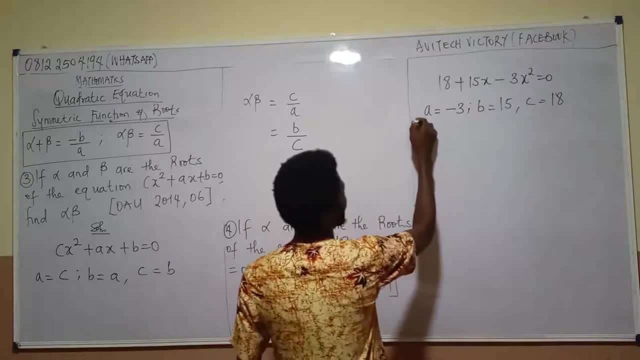 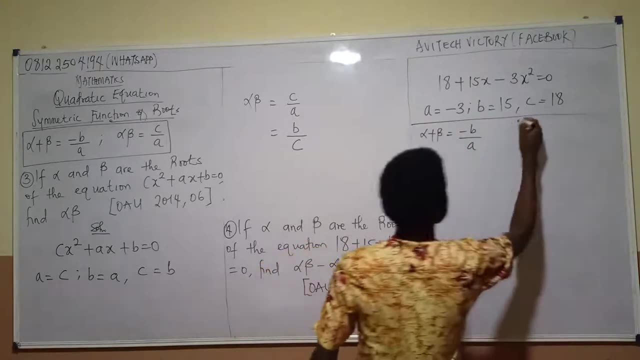 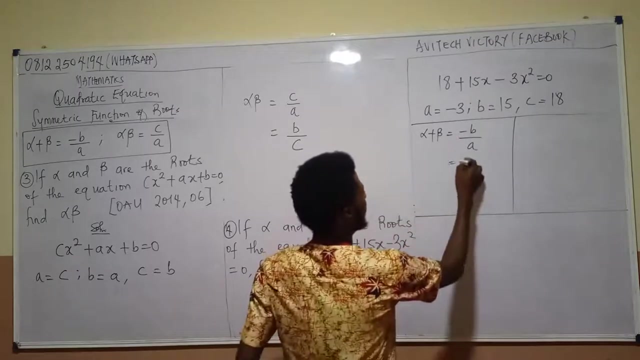 you find alpha plus beta. So alpha plus beta. I told you it's minus B over what A. That's alpha plus beta. So alpha plus beta is minus B over A. So this will now become minus what is B? What is B? 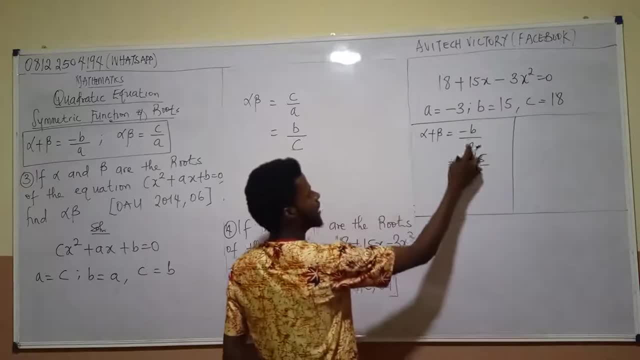 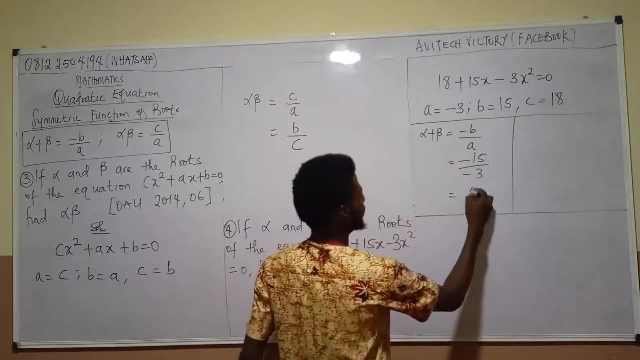 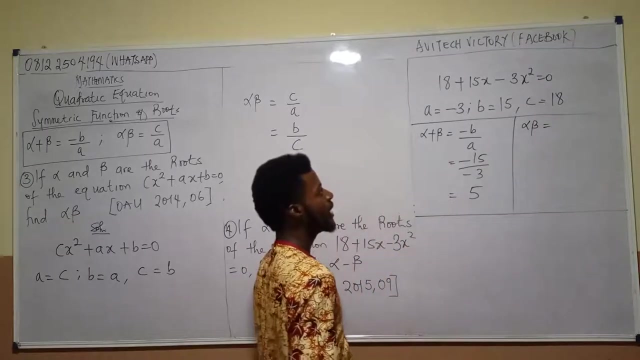 B is what 15 over what is A. A is what Minus 3.. So if we check this out, minus 15 divided by minus 3 will give me 5.. Then the next part is alpha beta. So what will become alpha beta? Alpha beta is C over what A In the formula. Remember I said: 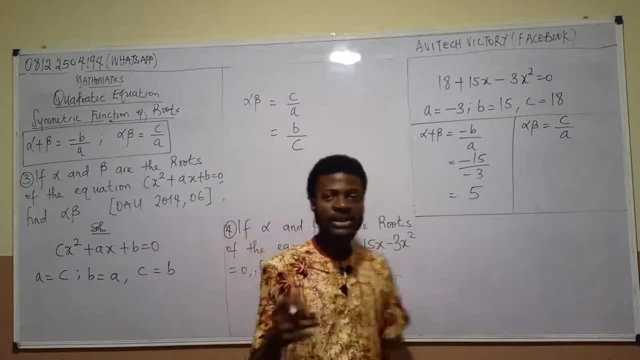 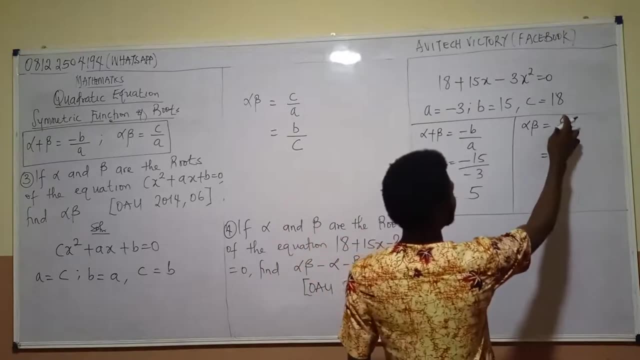 take note of this. It's very important. Take note of that. It is very, very important. Okay, So alpha beta is C over A. So what is C? C is what. 18 divided by what is our A? A is what. 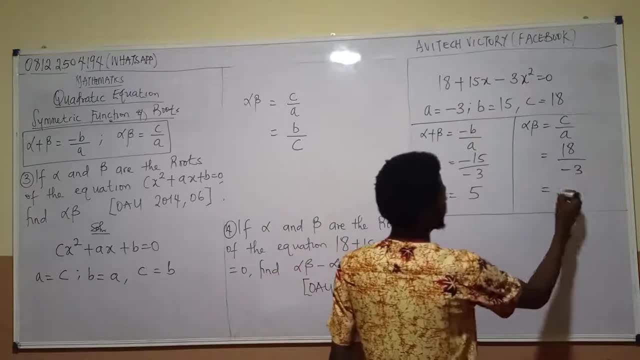 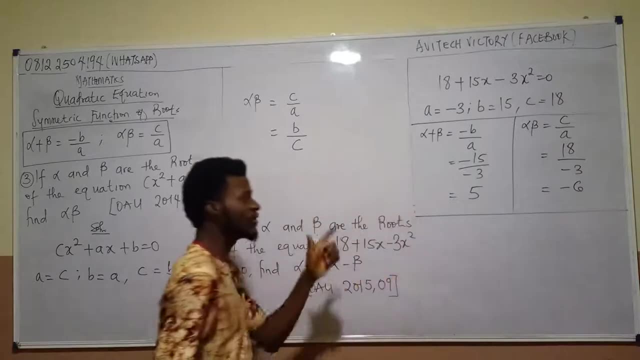 Negative: 3.. So what do you think this will give to us? Negative what? 6.. 18 divided by 3 is 6.. Then put a minus sign. So if that is what we have, alpha plus beta is 5.. Alpha beta is minus 6.. 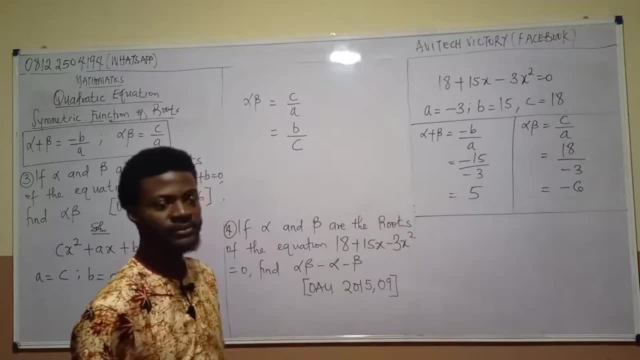 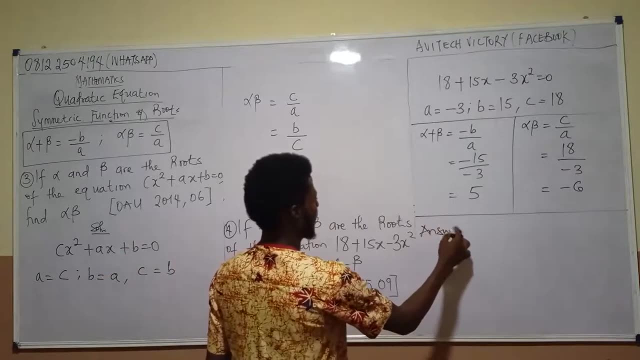 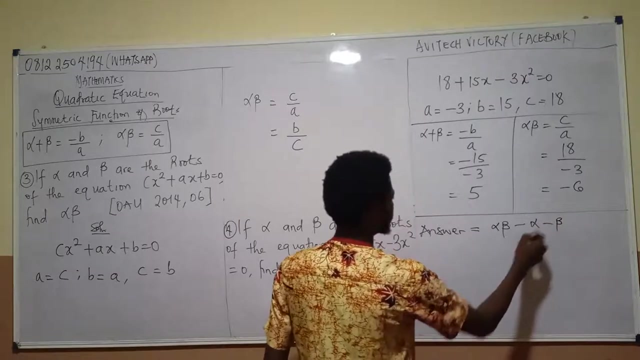 How do we then solve this question Now? the next thing is, let us then write what they ask us to find. So the question says we should find the answer of alpha, beta, take away alpha, take away beta. Now, if you look at what the equation says we should find, if you look at it properly, you'll 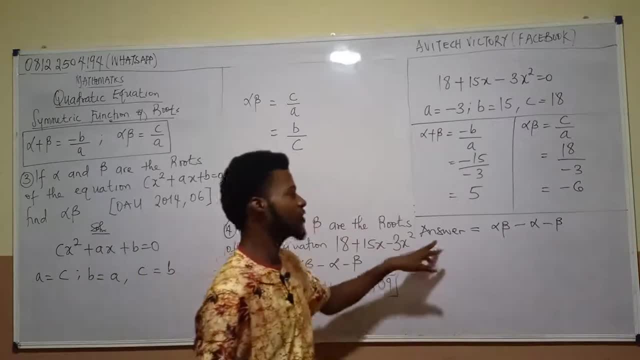 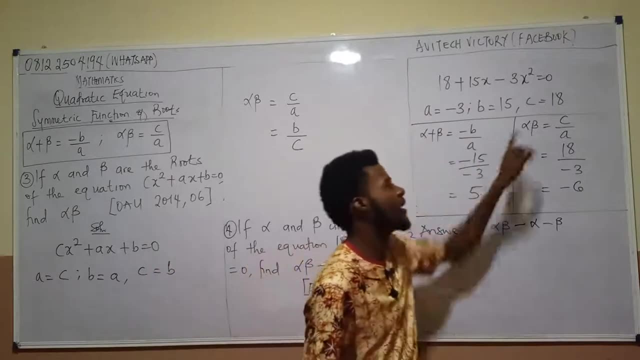 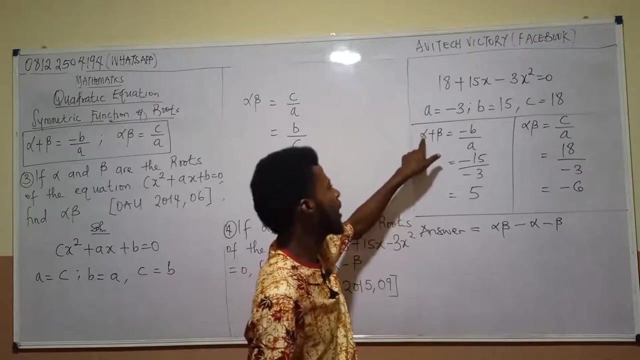 notice something, Remember? I said you must try to make this very guy look like alpha plus beta and alpha beta. That's what I said. You must try your best to make sure that the expression is going to have alpha plus beta and alpha beta. So right now, how do we make this expression have these two things? 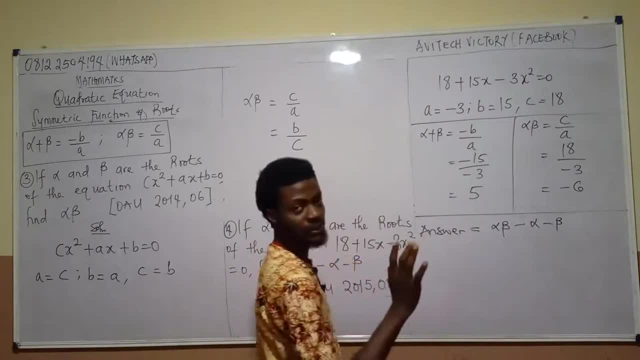 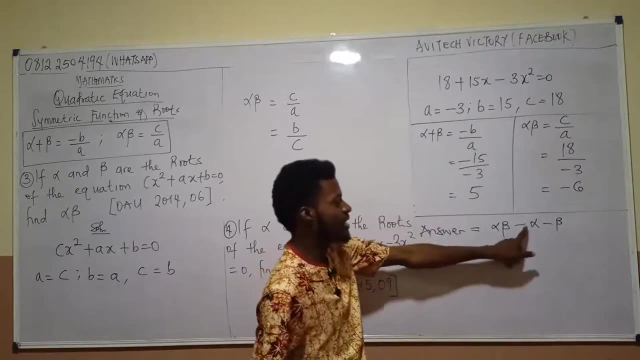 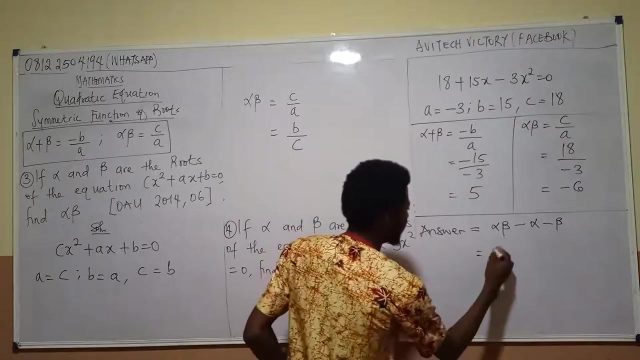 Take note: Alpha beta is already settled. Alpha beta is already what Settled. But we have an expression. It has minus alpha, minus beta. So how do we make minus alpha, minus beta become this? Now look at this, This alpha beta, I have the minus sign common between these two guys. I have the